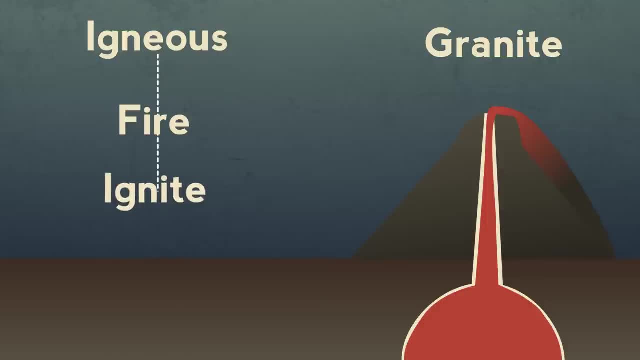 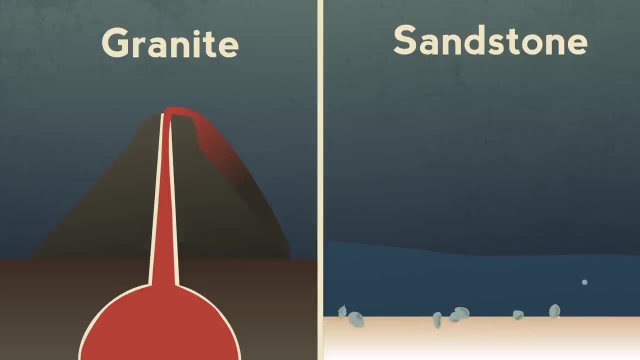 rock In the Latin word meaning fire- Think of the word ignite. But sandstone was made by bits of other rock carried by rivers to the sea. The bits get smoothed and rounded like the pebbles on a beach. These grains settle on the seabed, forming sedimentary. 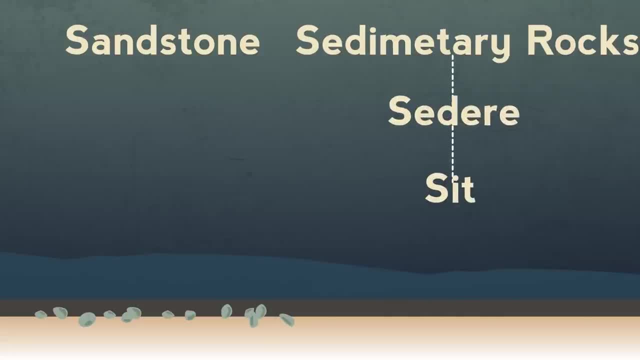 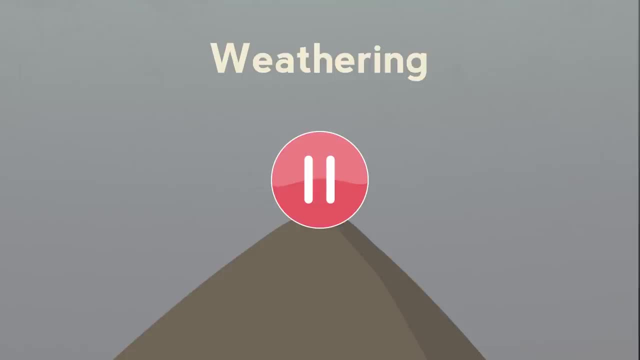 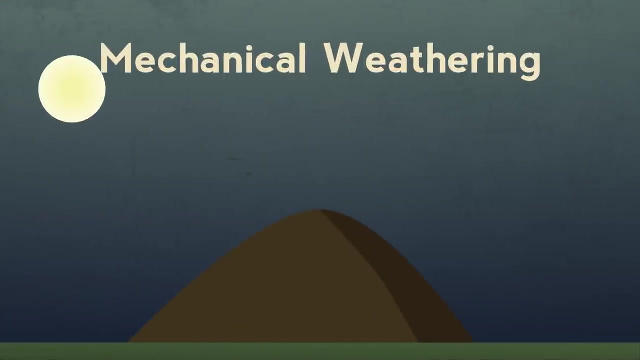 rocks, From Latin sedere to sit. Rocks get broken up by a process called weathering. Pause and think what sort of weather might break rocks. Mechanical weathering: The heat of the sun expands the rock. It contracts at night, causing 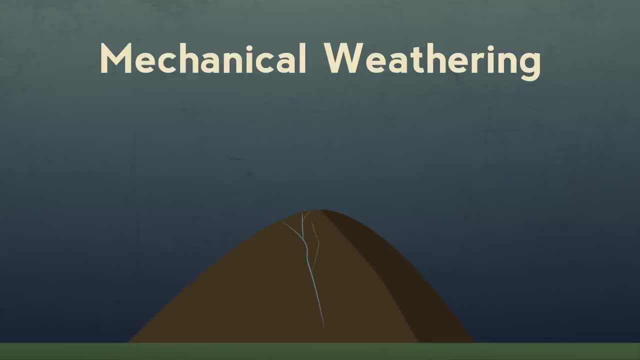 it to crack. If water enters and freezes, it will crack more. With water and wind, bits of rock knock into each other, breaking them. Chemical weathering is when rain, which is slightly acidic, dissolves some minerals in the rock. 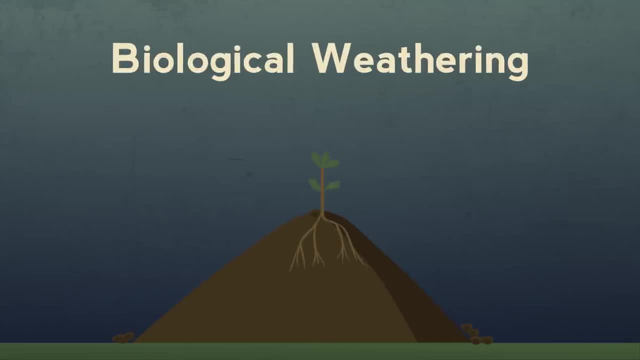 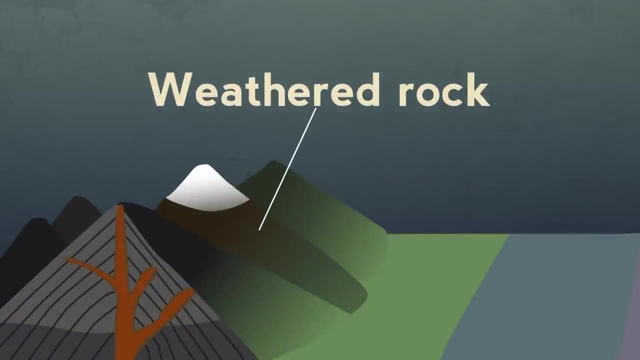 Biological weathering happens as lichens and then the roots of plants grow on the rocks, forcing their grains apart. Weathered rock forms the soil, but it is also eroded. that means transported either by wind or, more usually, by water to the sea. 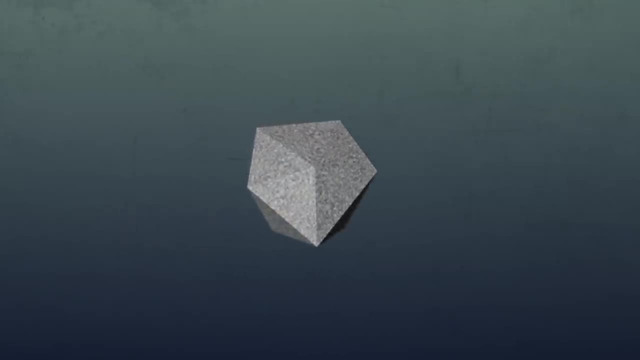 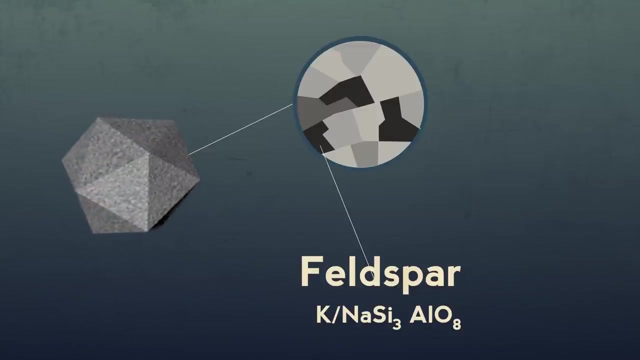 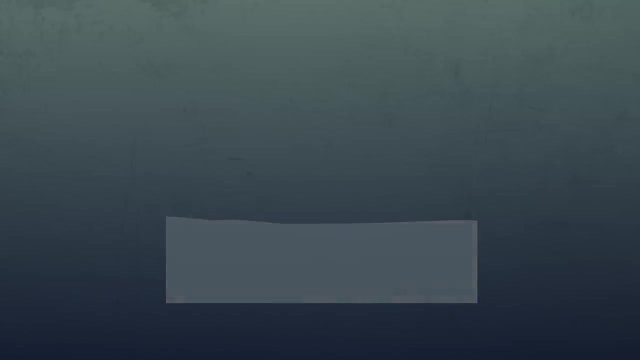 Notice the dark and light-coloured grains in granite. These are minerals, the pure substances that make up rocks. The dark grains are feldspar And the light grains are quartz. After weathering, the grains are carried to the sea, where the harder quartz settles. 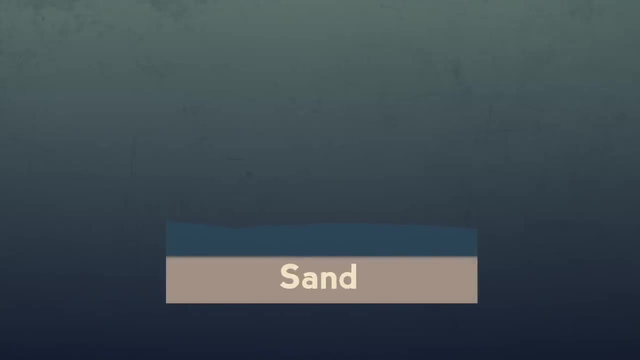 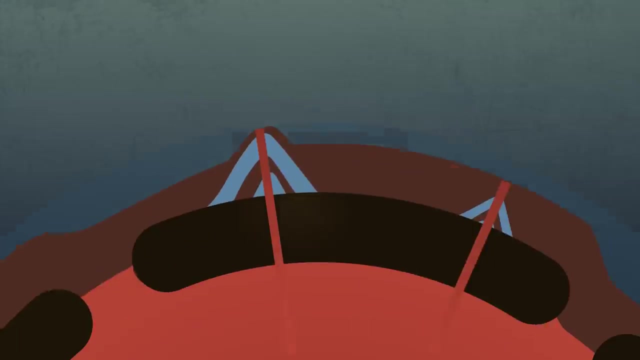 as in a jar of soil, forming sand. The feldspar settles more slowly, forming rich beds of clay containing most of the trace metals plants need to grow. During the movement of the great tectonic plates, the rocks get folded and squashed, often ending up high in the air. as do the rocks. 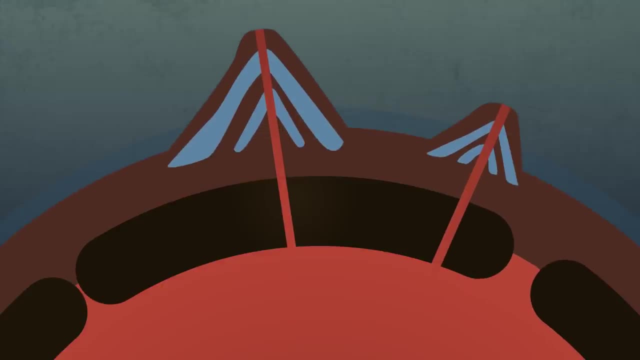 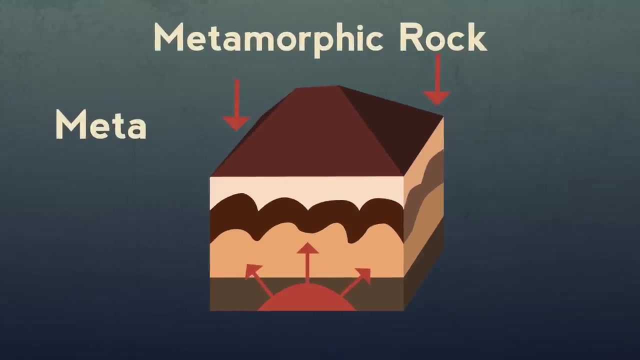 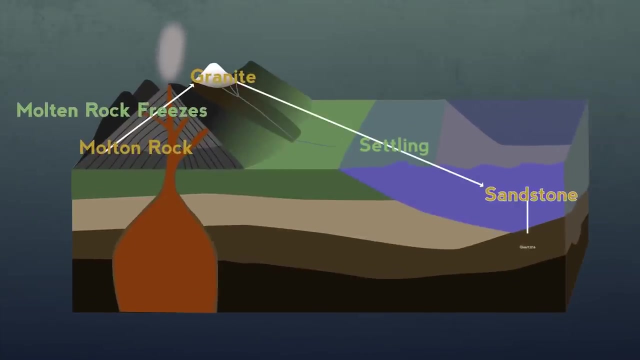 The rocks get folded and squashed, often ending up high in the air, as do the rocks. The rocks get folded and squashed, often ending up high in the air, as do the rocks. These rocks are called metamorphic rocks. From sandstone we get quartzite and from clay we get first shale, then slate. 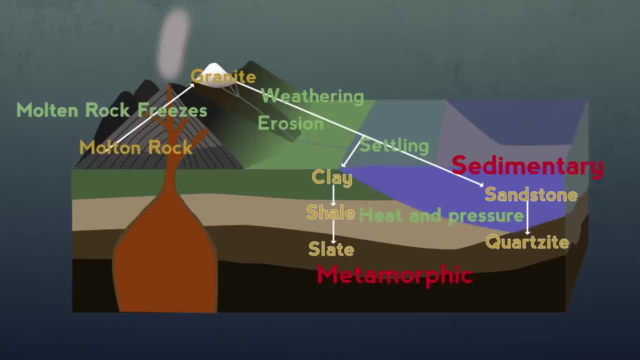 Sedimentary and metamorphic rocks get weathered and eroded too. Tectonics carry the rocks down into the Earth's hot mantle, into the sea and into the earth. They get heated in time for the next 30 minutes or until the rocks have formed.